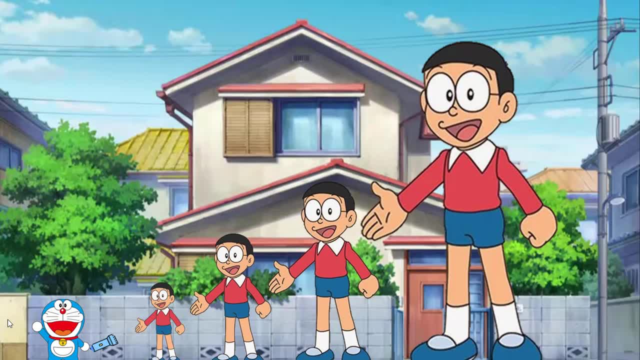 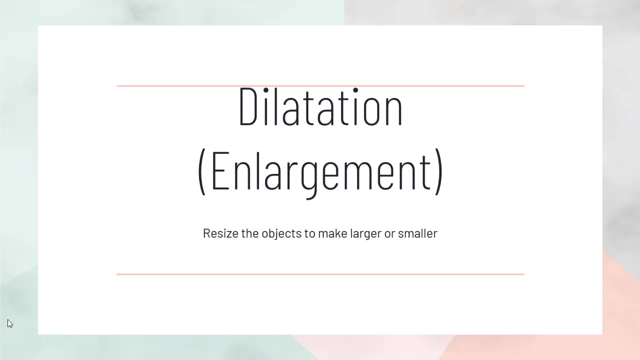 bigger, bigger and more bigger. Wow. So right now we know the function of this flashlight: to make someone or an object to be more bigger. So basically, this is the illustration of our lesson today about dilatation. So dilatation or enlargement have a definition: resize the. 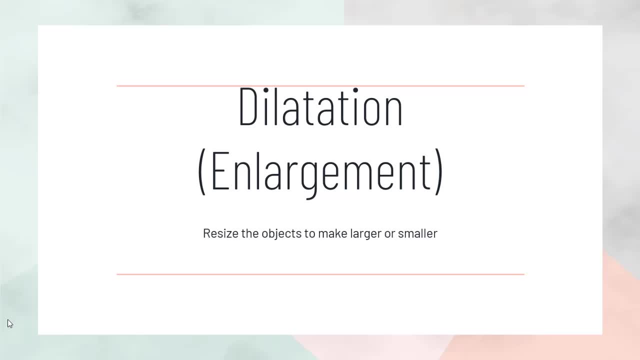 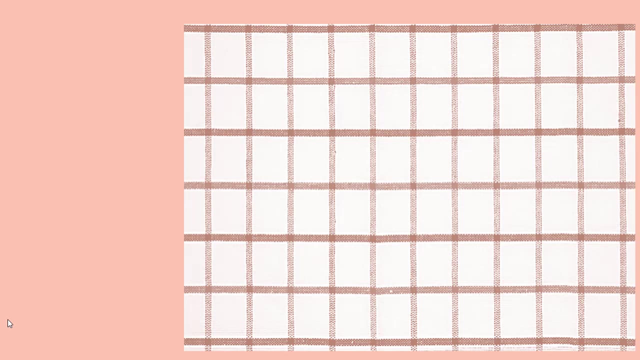 object to make it larger or even smaller. So to give you an idea about this concept, let's we check the illustration. Okay, this is the illustration, so I borrow Doraemon's magic flashlight. I'm gonna try to reside my small pizza here to make it more bigger. 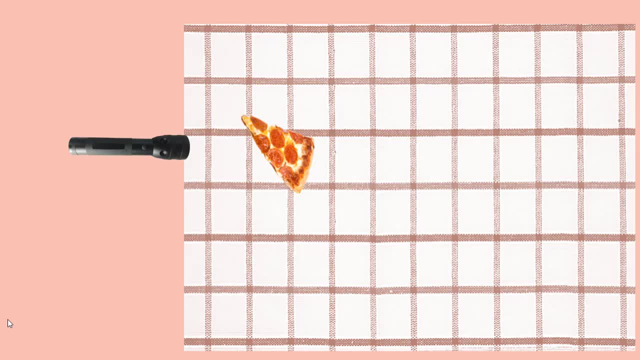 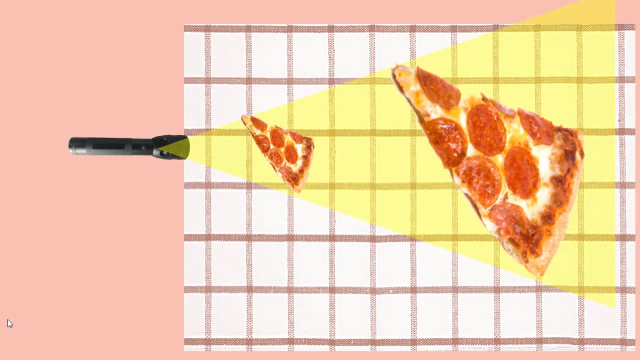 So look at this: I want to make my pizza three-more bigger using Doraemon flashlight. So look at this: wow, my pizza is getting bigger. So I will enlarge my pizza three times more bigger so that the center of flashlight is O to make the middle one bigger. So I so that the center 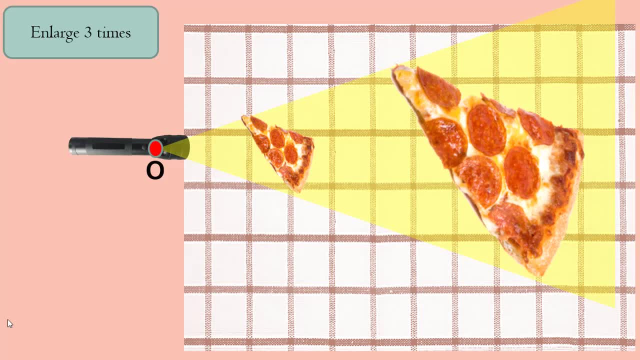 of the flashlight is O, to make the middle one bigger, or center of the dilatation, and left the pizza is a triangle with the vertex A, B and C and my big pizza A accent, B accent and C accent. so because before I told you I want to resize my pizza three more bigger, three more larger, so that's mean. 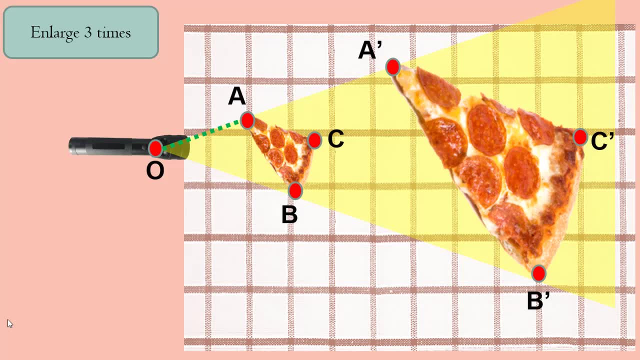 Oh, to fight Oh a accident, we have to multiply three times Oh a, because I resize the small pizza three times. then it's also same to find Oh the accent, to find the length of all the accent. so you have to multiply Oh B times three because I resized. 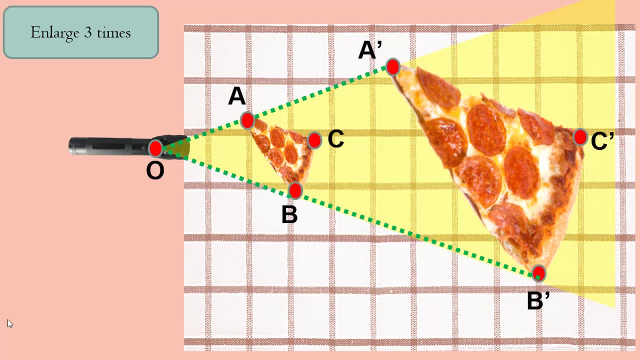 may be zot three times and also, as will be the same with Oh C accent, you have to multiply three times Oh see, to get Oh she acts in. so that's mean Oh a accent is equal three times Oh a, Oh B accent is equal three times Oh B and then Oh C. 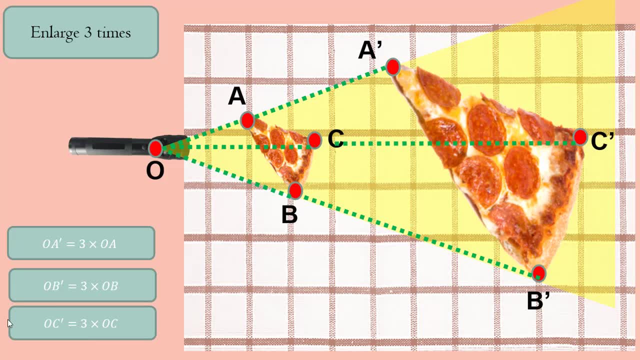 accent is equal three times. um, Ohそうだ, I thought. oh, my guess. and so we need to normalize the power of all the OC, or we can find the ratio of the distance, which is OA. accent out of OA is equal OB. accent out of OB is equal OC. accent is out of OC is equal 3. so this is 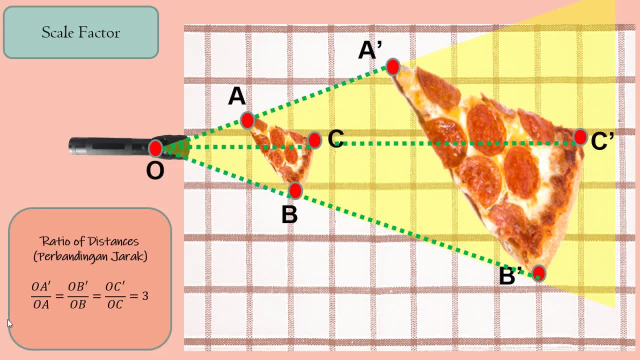 we call scale factor. so scale factor have a definition: the size of an enlargement or reduction. dilatation is not only about make an object more bigger. sometimes it makes an object more smaller. now we will learn together how to find the ratio of the distance, between the distance, between the distance and the. 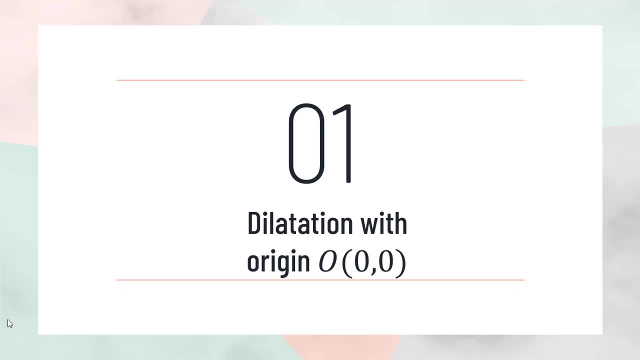 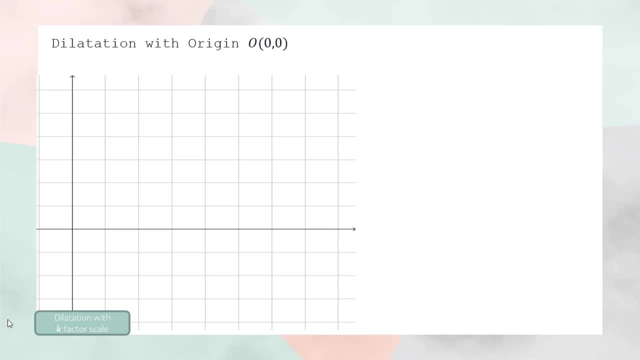 coordinate of the image onto dilatation. so the first about dilatation with the origin 0,0. okay, I have a Cartesian coordinate here with X and Y axis, and if I have an origin point or center of dilatation- 0,0- and there is a, 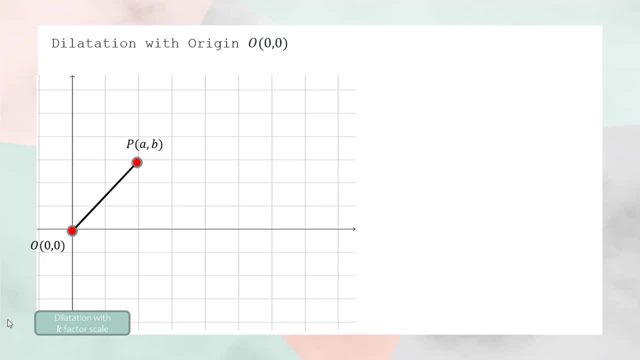 point B, and now we have to connecting O and P will be the line segment OB, and let's define all the properties of point B vertically and horizontally. so length of O to P horizontally is a units and then length of O to P vertically is B units. 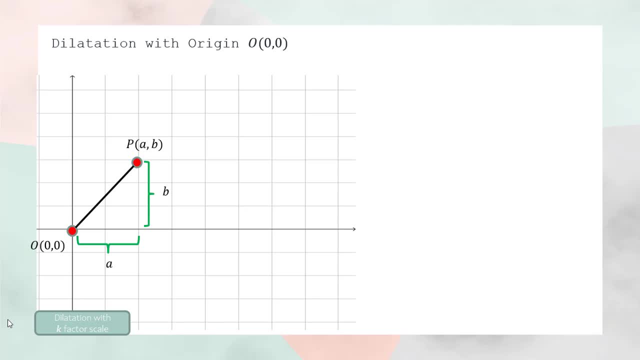 and now we can sketch the right triangle, triangle of all this side. So the pink triangle with the hypotenuse is OP and with the leg A and B. And if you want to dilatation this right triangle more bigger, 3 times with k. 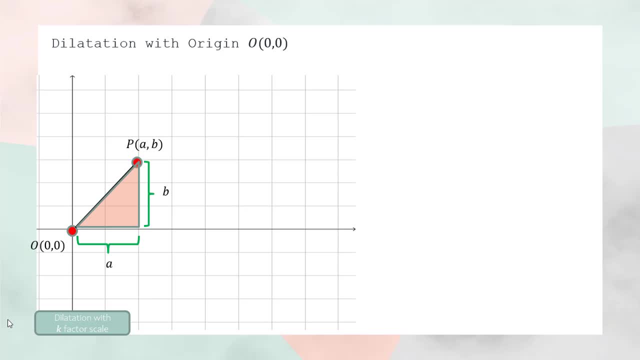 vector scale. So the leg of the big triangle will be k times more bigger than the previous leg, so k times A, And then for the other leg we also have to multiply with k And then we can sketch a big triangle. after we dilatation this, more triangle. 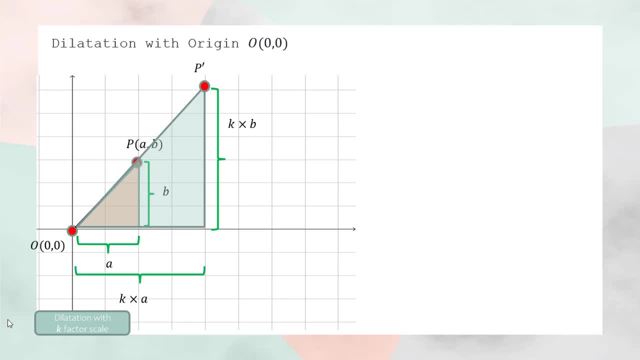 So the new hypotenuse of this big triangle under dilatation is the OP accent. So OP accent is equal to k times OP. So we found the formula for dilatation with origin O, with the coordonate A, B, when. 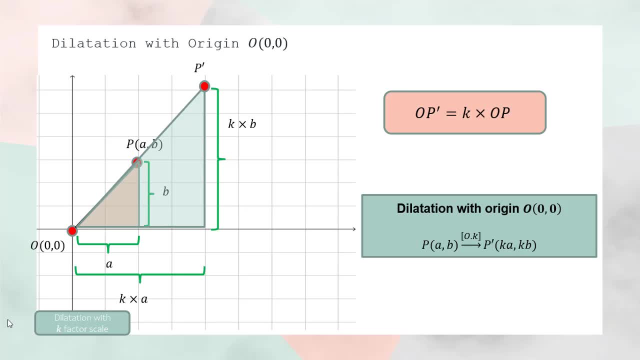 you dilatation with the origin and the scale factor k, so you just need to multiply all the coordinates kA, kB. It's easy, right? So to give you an idea about this formula and how we use it, let's do an exercise together. 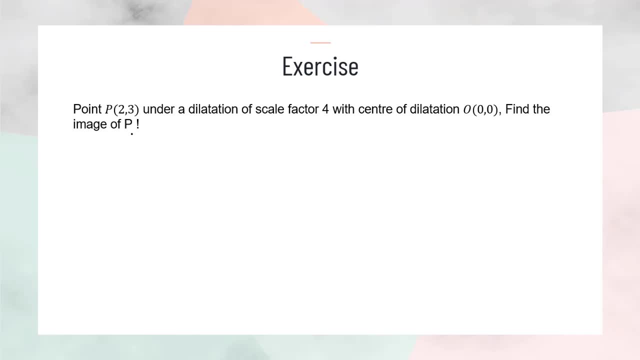 And I have a question here, Remember point P, with the coordinate 2,3, under dilatation of scale factor 4, with the center of dilatation 0,0, and we have to find the image of P, or which is, we have to find the P-accent. 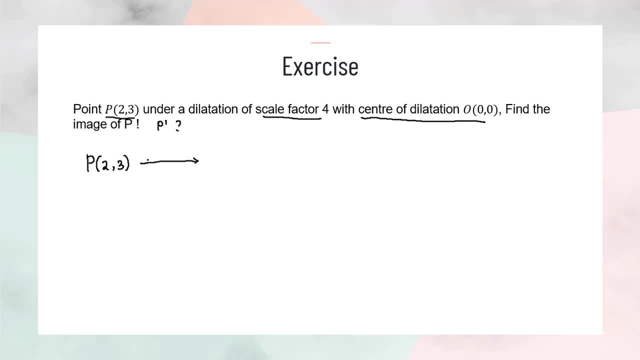 Are you still remember the formula of dilatation with the center of dilatation 0,0?? Yep, Okay. P with the coordinate 2,3.. Under dilatation with the origin point 0,0, with the factor scale 4.. 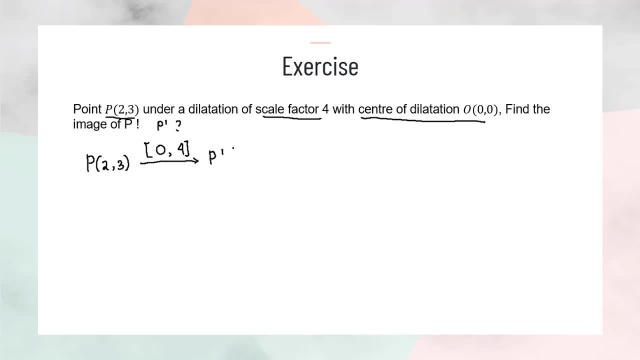 So to find the P-accent we have to multiply all the coordinate x-axis and y-axis with 4.. Because 4 is the factor scale, so 4 times 2,, 4 times 3.. So the coordinate for P-accent will be 8,12.. 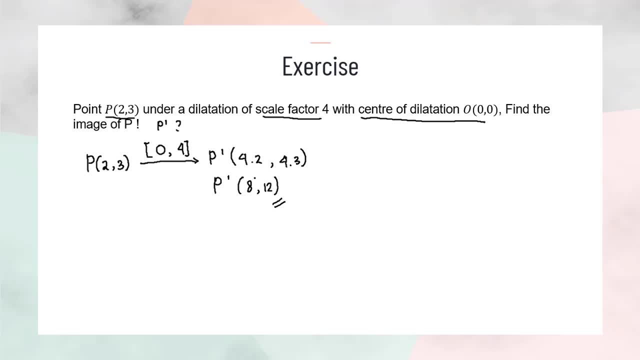 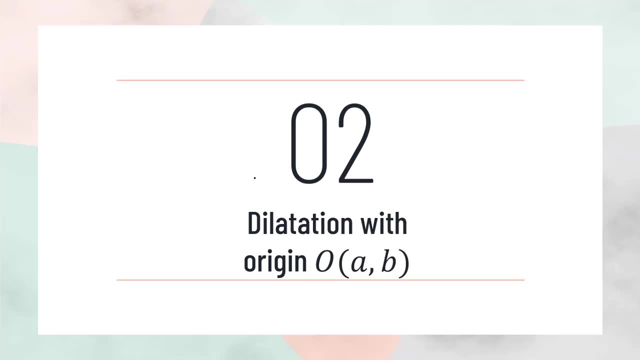 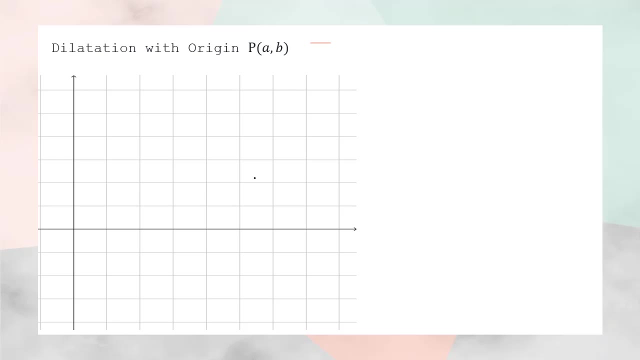 It's so easy, right? And now let's move on to the next dilatation, about dilatation with the origin 0, ap. Okay, to give you an idea, we'll sketch it on Cartesian coordinate with x-axis and y-axis. 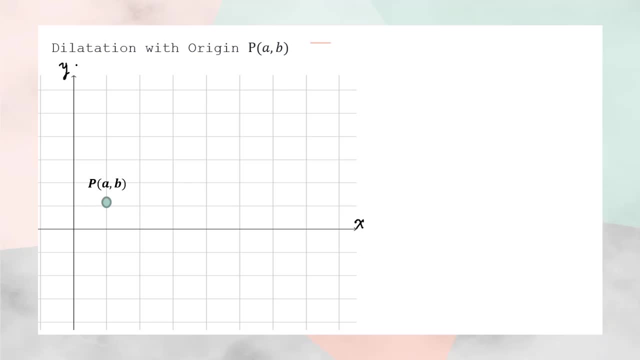 Well, if I have a point p with your coordinate a comma b, so for the length horizontally, the length of horizontal is a units and vertically is b units, and we want to find the image of a point which has a coordinate x comma y, why, under the dilatation p, a comma b, with k vector scale, again connecting p and a with the line. 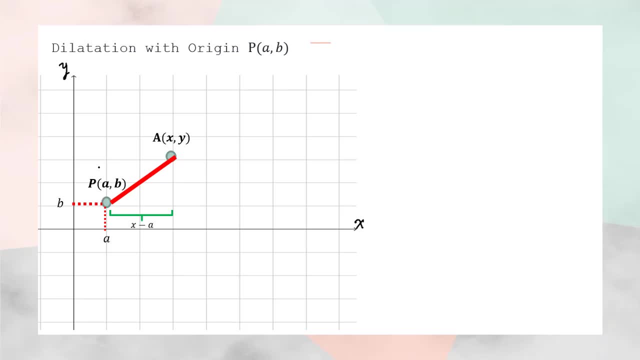 segment. and now we have to find all the properties of point a vertically and horizontally. for horizontal with b, x, and for vertically will be y. so the length from the center of dilatation will be X minus A, and then vertically from point P, which is center of dilatation, will be Y comma P. now we can sketch the right triangle. 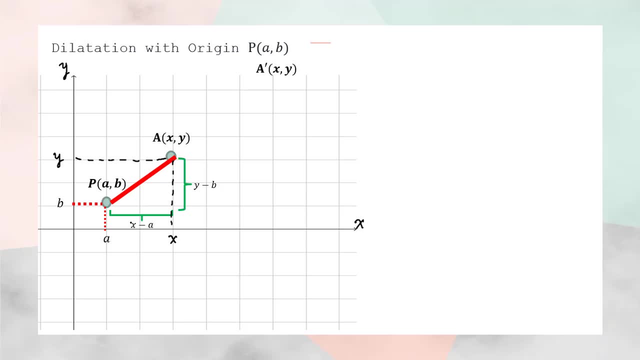 of all, the side with the hypotenuse is PA, with the lag X minus A and Y minus P. so this is a triangle. and because we want to resize this triangle more, bigger, K times with the vector scale. so the leg of the triangle will be three more. 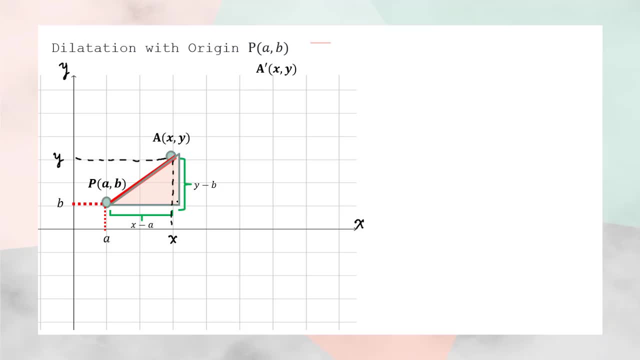 bigger than the small triangle. so it will be for the horizontal one K times X minus A, then for the vertical one, K times Y minus B, and then we can sketch a big triangle after we resize the small triangle to be more bigger using all the lag. so this is a big triangle after we resized and we can find the length of PA. 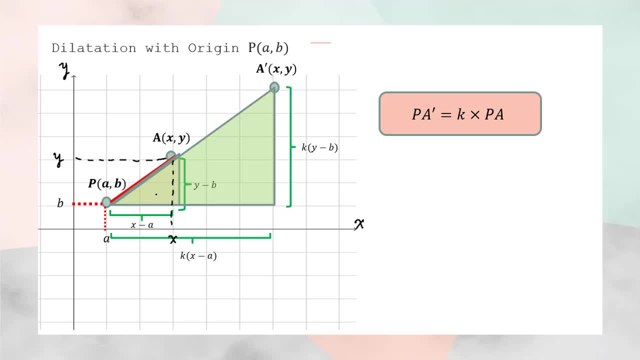 accent will be K times PA. so this is the formula after dilatation. so if we have a point A with the coordinate X comma B and we dilatation this point A comma B with the K factor scale, so we can use the formula for a accent. 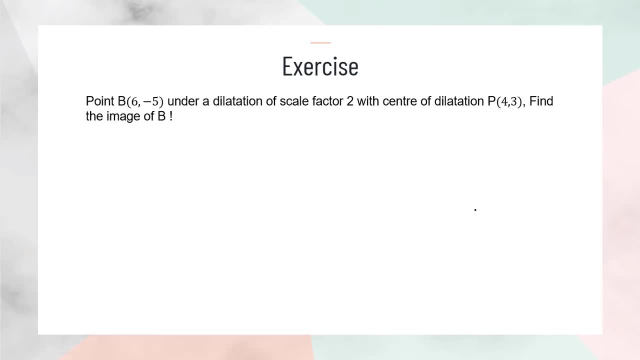 well, to give you an idea about the formula for A accent, you can use the ID about the formula. let's see another one such auled. I have equation point B, 6 comma minus 5, under a dilatation of усcali Dahua I2 and with the center of dilatation with the point P, 4 comma 3. we. 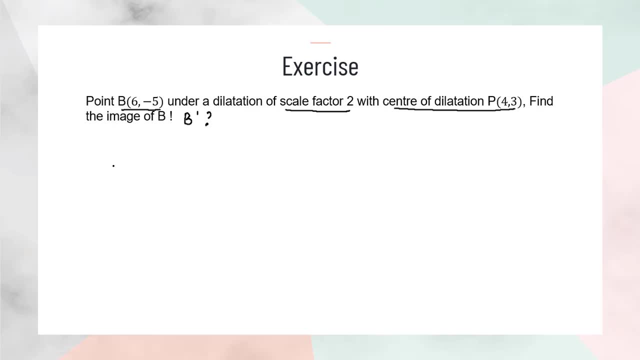 have to find the image of D, which is the accent, is to remember what the formula I gave. I have point D which have a coordinate 6 comma minus 5 and really light hatred. I'm serious, guys, if you make fine Prem so lukewarm stress. C to the ac GP местur. 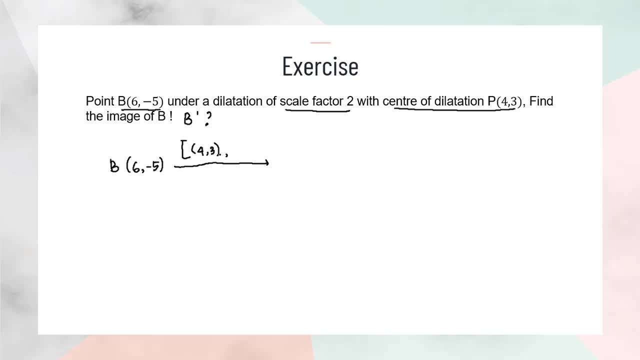 with the center 4,, 3, and then with the scale factor 2, and we will find the accent which have a coordinate x-accent, y-accent. and I used to remember the formula for x-accent: yeah, correct, k times x-a plus a. so 6 is for x minus 5 for y, 4 for a, 3 for b. so 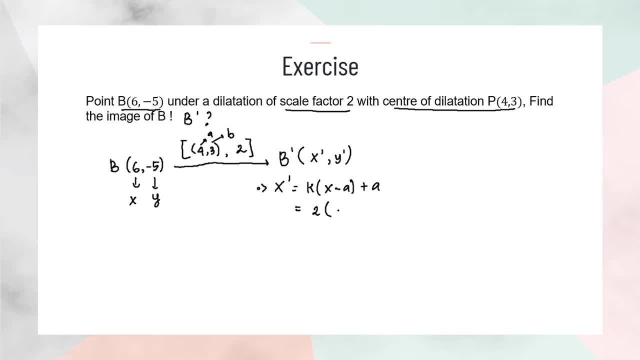 we can do. substitution for k is equal to 2 times 6, 4 plus 4, so 2 times x-accent times 2 plus 4 is equal 8, this is only for the x-accent. now we have to find for the. 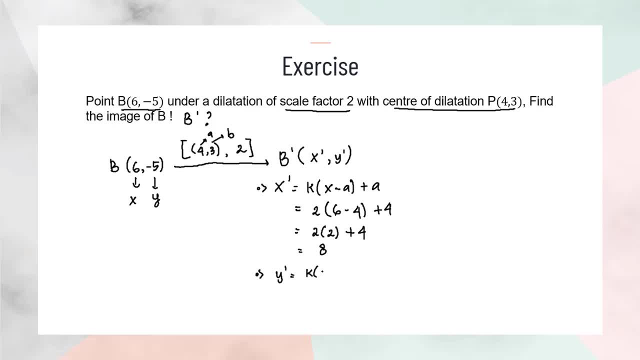 y-accent. so y-accent is equal to k times y b plus b, and we can do substitution using a formula: it's equal to minus 2 times minus 8 plus 3, so it's equal to minus 30, and 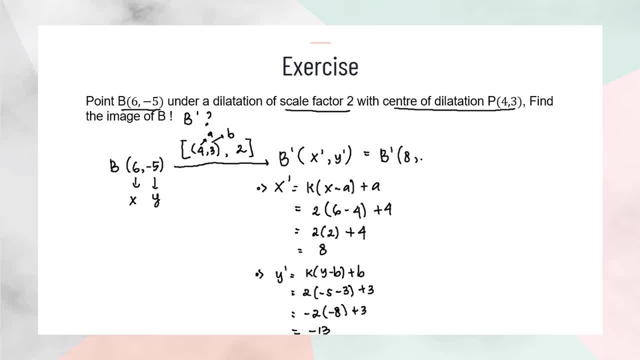 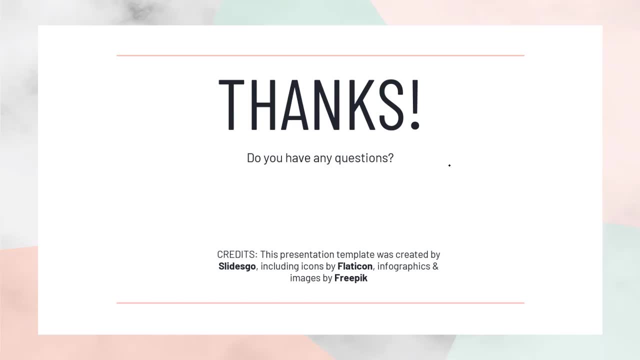 the coordinate of b-accent will be 8, minus 30,. it's easy. you can try it at home. okay, that's all for our lesson for today. I hope you enjoy and see you on the next video. goodbye.